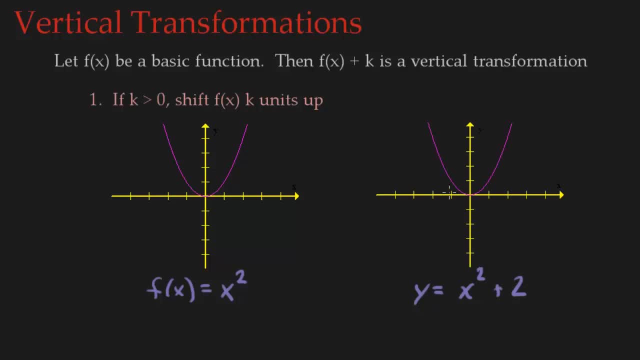 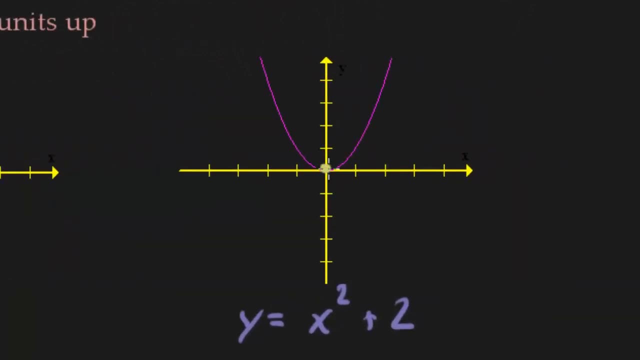 Let's go ahead and graph that. So let's take every point on my function and shift it up two units. So I have this point right here, right there, We will shift that up two units. So everything else just goes up two units. So here is the point one, one which is now up at one three, The point two. 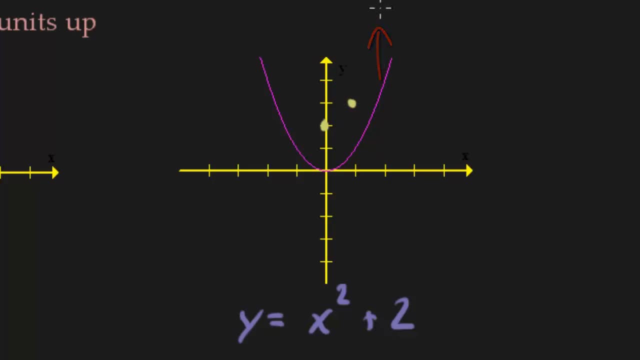 four is now going to be up at two six. So that is off the graph, but it will be somewhere right there. Negative one one will now go up to negative one. It will go up two units, One four. negative one, I'm sorry. negative two four will go up to negative two six. And when we 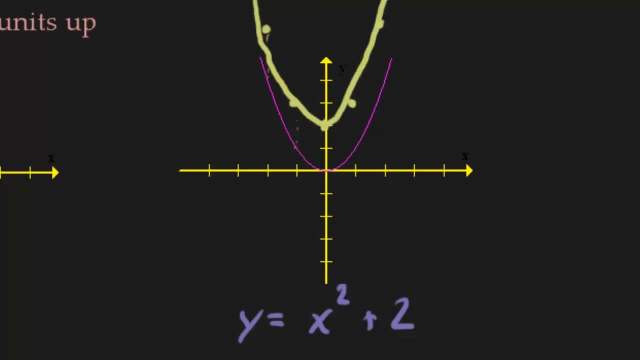 connect them. that's what we get. Since that picture didn't look too good, let's let me just graph it one more time. Still looks the same. Notice that your graph has been shifted up twice. So this point went up. two units went up two units here went up two units. 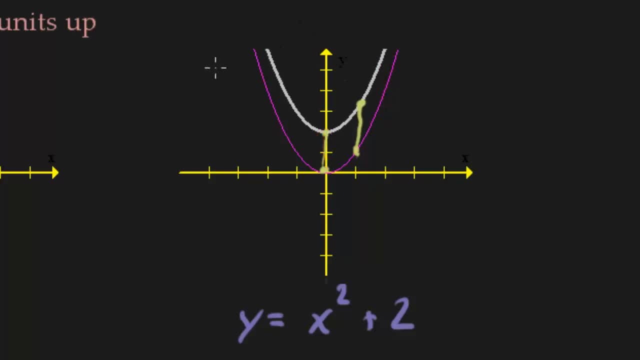 So this is my new graph right here. All right, So this is a vertical transformation. When I go up, let's go ahead and shift down. Now, if k is less than zero, we're going to shift our basic function k units, down. So that would. 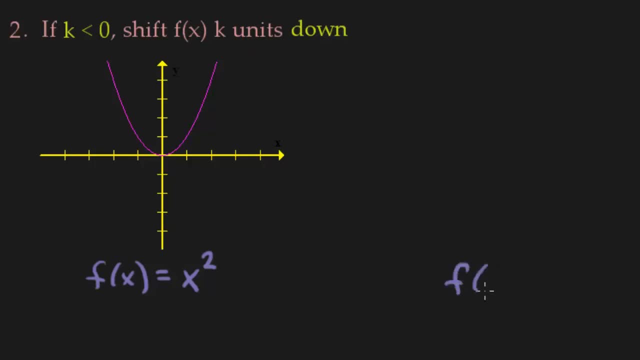 look something like this: Let's take f, let's do it like this: Y equals x squared minus, and I guess we could do minus three. So this is going to be a vertical transformation. it's going to be a shift down 3 units, because k is negative 3, so down 3 units. So there's. 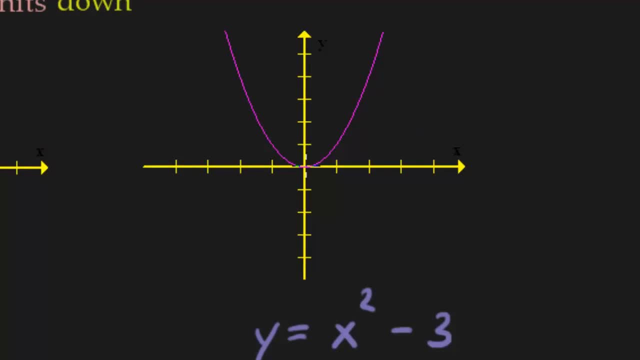 our basic function. Let's just move everything down 3.. So this point right here down 3, that's my new point: 1, 1, we go down 3, right there, 2, 4, we go down 3, puts me at 2, 1.. 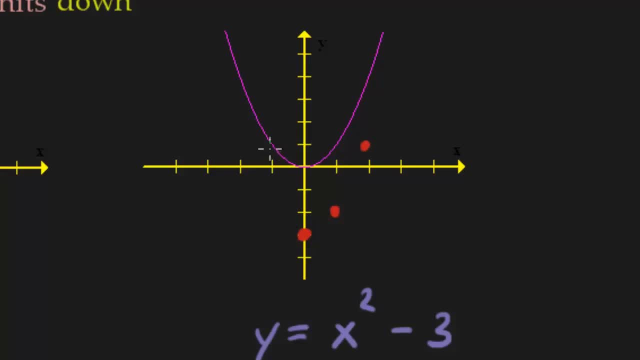 Over here down 3,. so if we're 1, negative 1, or, I'm sorry, negative 1,, positive 1, we go down 3, puts us here. Negative 2, 4, we go down 3, puts us right there. So what I'm?